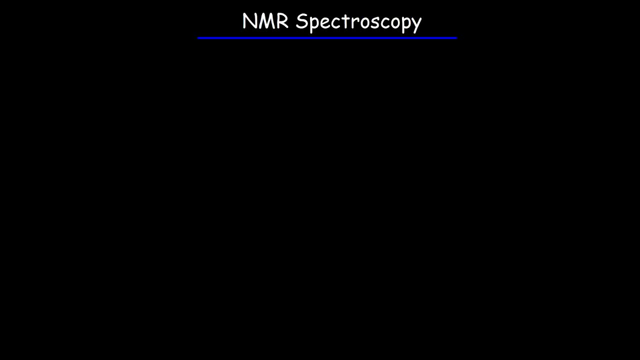 In this video, we're going to talk about the basics of NMR spectroscopy. NMR spectroscopy is useful for identifying the carbon-hydrogen framework of an organic compound. Now it only works with certain nuclei, and that is nuclei either with an odd number of protons. 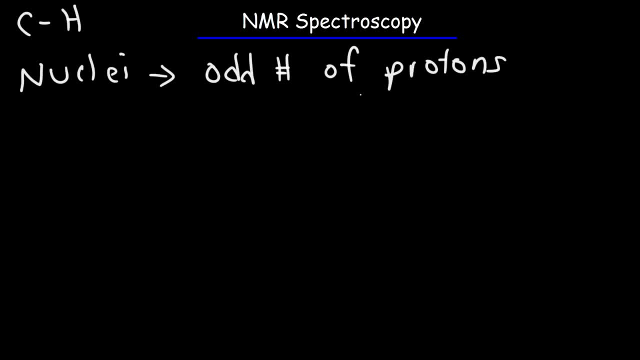 or an odd number of neutrons. So let me give you some examples. So nuclei such as hydrogen carbon-13,, nitrogen-15,, fluorine-19, and phosphorus-31,. these nuclei either have an odd number of protons or an odd number of neutrons. 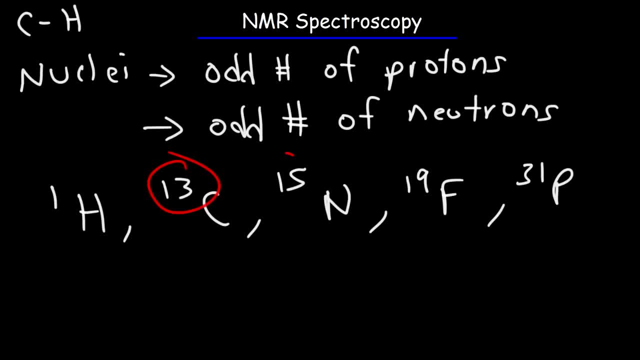 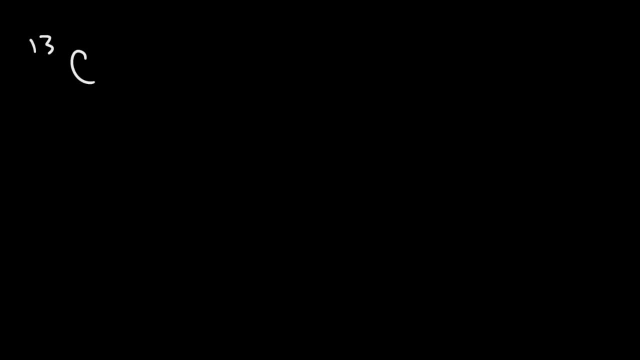 Because, as you can see, the mass number are all odd And the mass number is the sum of the protons and the neutrons. So let's take a look at carbon-13.. So carbon-13 can work with NMR spectroscopy, but carbon-12 cannot. Every atom of carbon has an atomic number. 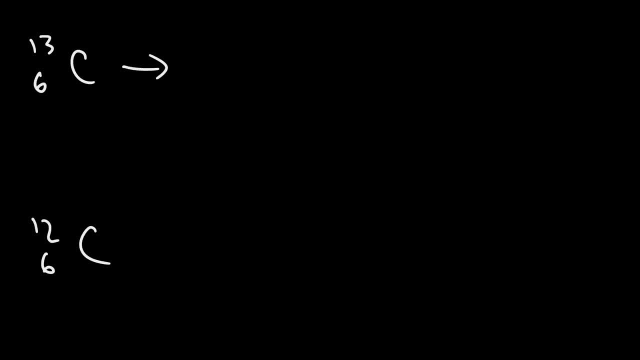 of 6. And, as you recall, the atomic number of 6 is the atomic number of carbon-13. So carbon-13 has an atomic number of 6. And, as you recall, the atomic number of carbon-13 represents the number of protons. So carbon-13 has 6 protons and 7 neutrons, The mass number. 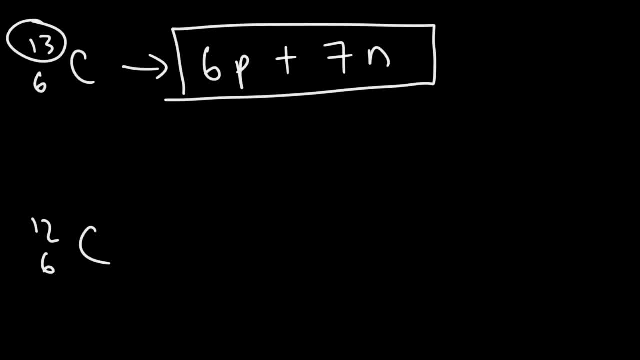 13 is the sum of the protons and the neutrons. Carbon-12 has 6 protons and 6 neutrons. Carbon-12 does not have an odd number of protons, nor does it have an odd number of neutrons. So 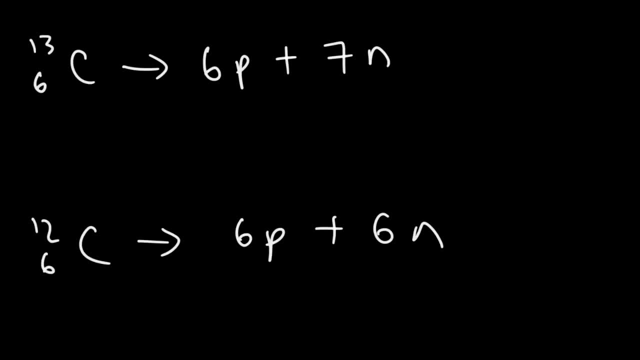 carbon-12 does not have a property called NMR spectroscopy. Therefore its nuclei will not be used in NMR spectroscopy. Carbon-13 has an odd number of neutrons, So therefore you can use carbon-13 in NMR spectroscopy. 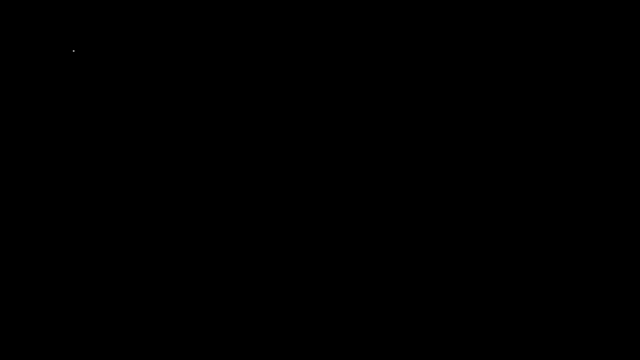 Now, before we go into carbon-13 NMR- typically you'll learn proton NMR or HNMR. Now, hydrogen has a mass of 1.. This is the most common form of hydrogen. There are isotopes of hydrogen, like deuterium and tritium, But we're going to talk about this particular hydrogen atom. 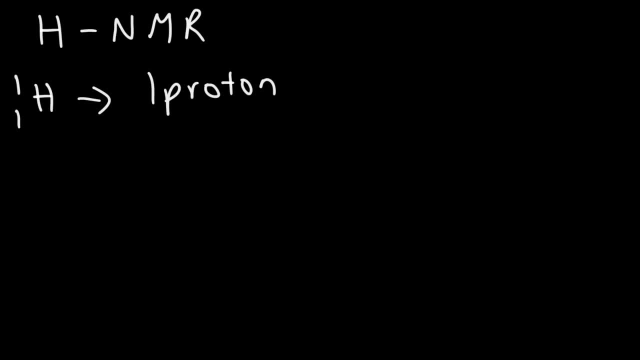 It has only one proton, no neutrons, So you can think of the hydrogen atom or the hydrogen nuclei rather as a proton, And a proton has a positive charge And it has a property called spin. And if you studied physics you know that. 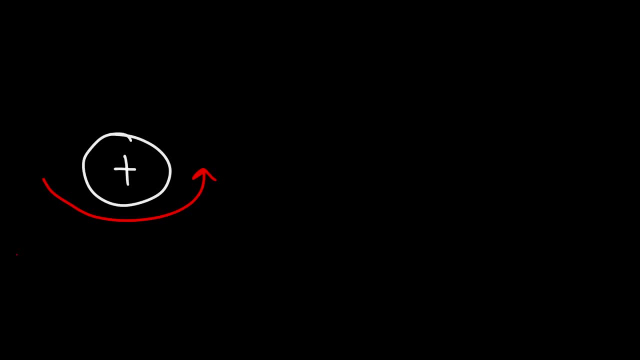 a moving charge creates its own magnetic field. So you can think of the protons as generating their own magnetic field. Now let's say, if we have a sample of protons, So these protons, their magnetic field, will have a random orientation. But what happens? 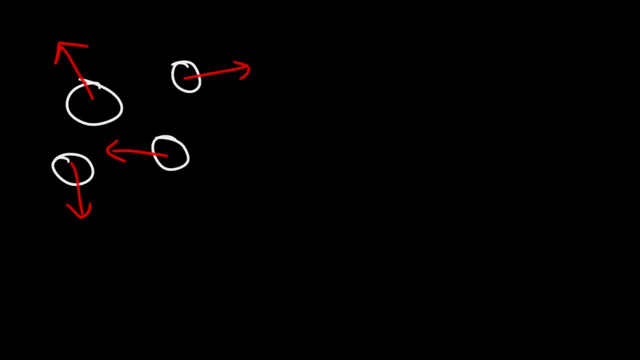 if we take these protons and put it in an applied magnetic field? What's going to happen? If we place them in an applied magnetic field? let's say it's going in the upward direction. we'll call it B-naught. Then the magnetic fields of the protons they could do one of. 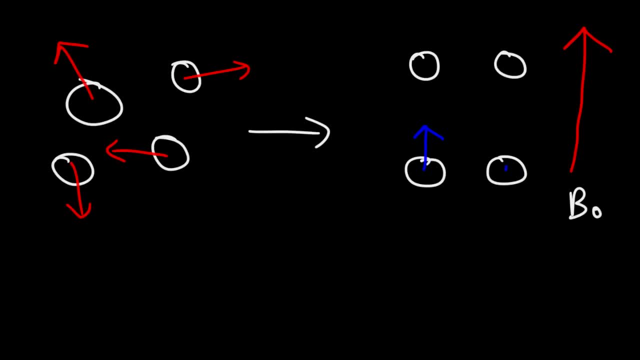 two things: 1. They can align. They can align with the external magnetic field or they can align against it. Whenever the nuclei are aligned with the applied magnetic field, this is known as the alpha spin state, And whenever they're aligned against the external magnetic field, this 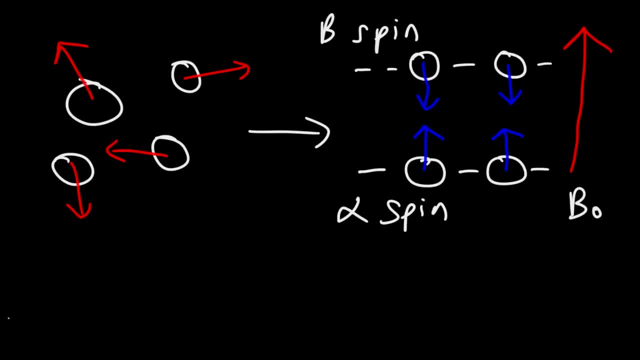 is known as the beta spin state. Now, as you can see, the alpha spin state is lower in energy than the beta spin state, And so the majority of the protons, or the hydrogen nuclei, will be in the alpha spin state, because it's more stable. And what helps me to remember? 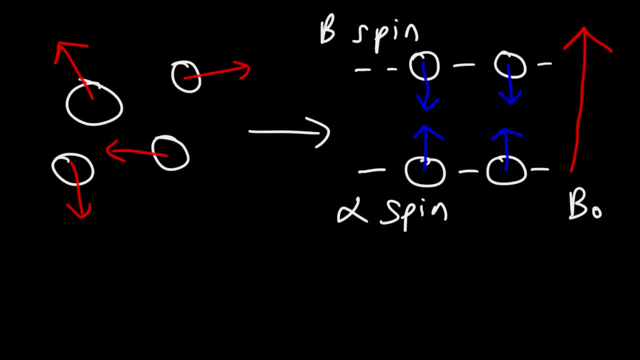 this is using the analogy of a river. It's easier to swim in the direction of the current rather than to go against it. So whenever the spin is aligned with the applied magnetic field, it's going to be in a more stable state. It's going to be lower in energy. 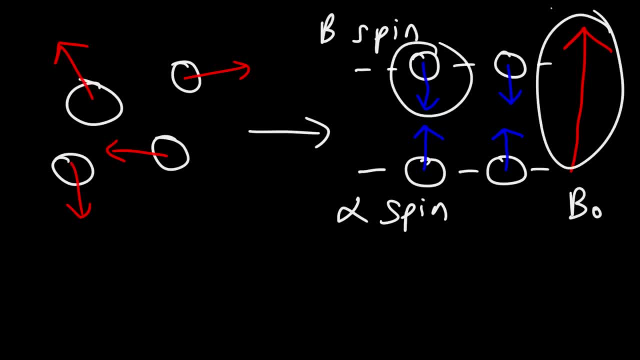 But it's going to be harder to go against the applied magnetic field, And so it takes more energy to do that. So thus it's in a higher energy state Now. delta E represents the difference in the energy of the alpha spin state and the beta. 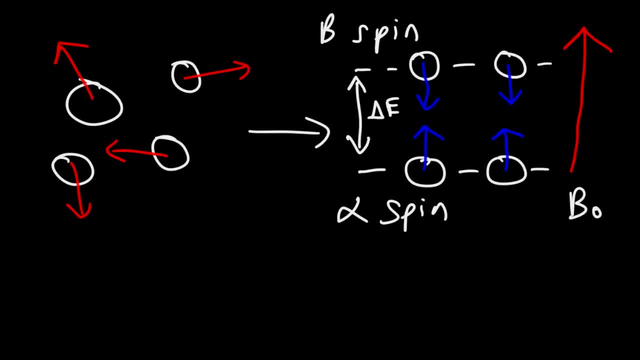 spin state. Now, the difference in energy is dependent on the strength of the applied magnetic field. So as you increase the strength of the applied magnetic field, delta E will increase, And so you're going to have greater separation between these two lines. Now, what does it take for a hydrogen nuclei to switch from the alpha spin state to the 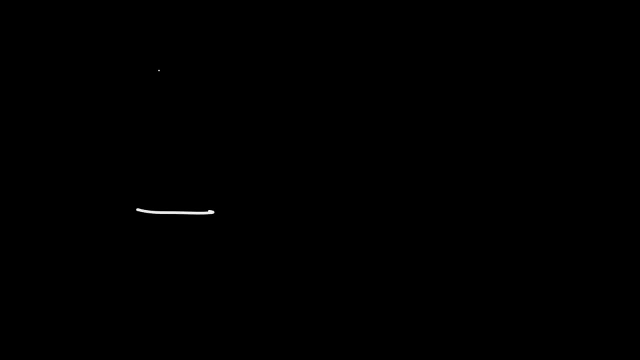 beta spin state. What you need is energy, particularly radio frequency energy. So if you add RF energy to a proton and if it's the right amount of energy, it can flip from the alpha state to the beta state. Now, if the nuclei falls back from the beta state to the alpha state, it can emit radio frequency. 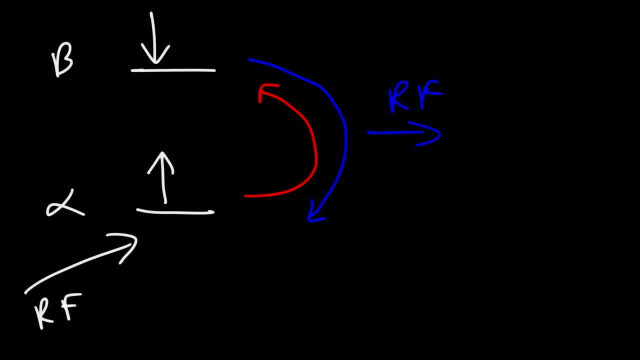 energy. But it takes radio frequency energy to promote it from the alpha state to the beta state, And so when it's constantly flipping back and forth it's in resonance. Thus we have the term nuclear magnetic resonance. So just remember that as you put energy into the hydrogen nuclei, you can promote it to. 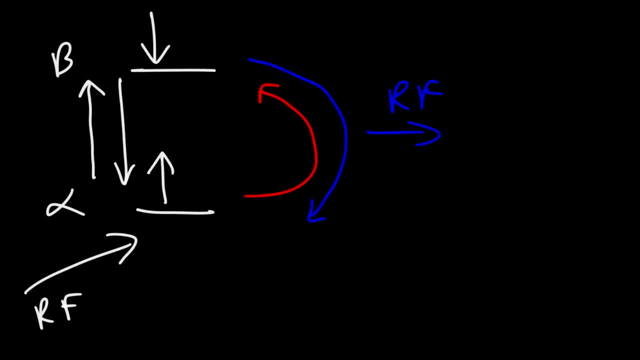 the beta state, And, as it falls back down, it's going to release energy. Now, if we want to, we can calculate the energy difference between the alpha state and the beta state, And here's the formula that we could use to do so. 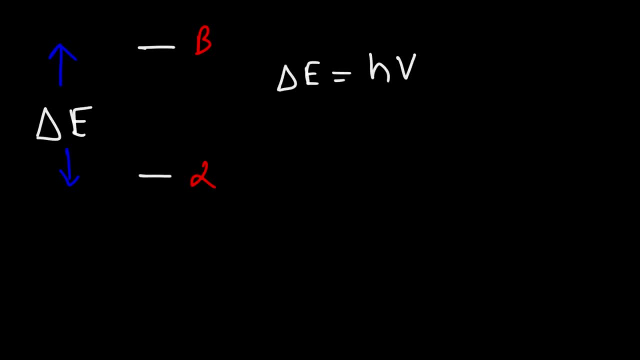 The energy difference is going to be Planck's constant times the frequency of the energy that we're going to use to put into the hydrogen nuclei. So we're going to use the energy constant times the frequency of the energy that we're going to use to put into the hydrogen nuclei. 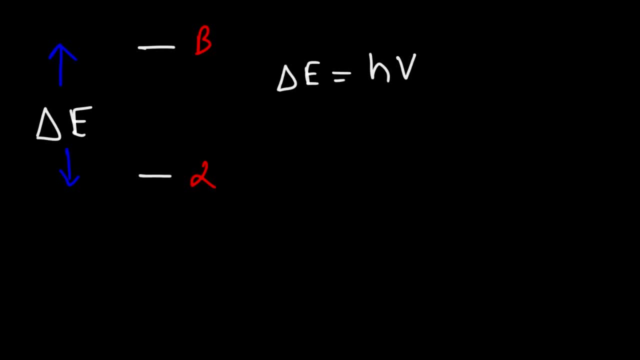 Put into the protons in the alpha state. Now the frequency that we need is going to be equal to the gyro magnetic ratio divided by two pi times the strength of the applied magnetic field, And so you could see that delta E, the energy difference between the two states, is proportional. 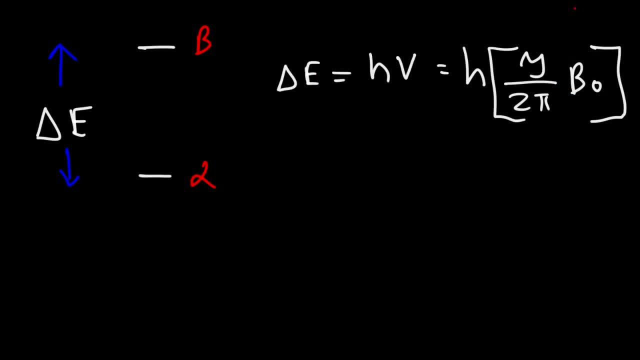 to the applied magnetic field. Now you might be wondering What? What is gamma in this particular equation? So this represents the gyro magnetic ratio of the nucleus that you're dealing with. So in the case of the hydrogen nucleus, the gyro magnetic ratio is going to be two point. 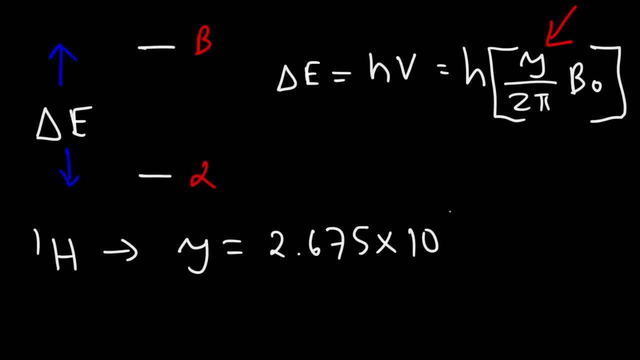 six, seven, five times ten to the eight. Tesla to the minus one times seconds to the minus seven. Now for the carbon 13 nucleus, it's different. It's going to be six point six, eight, eight times ten to the seven, And so it's less than that for hydrogen. 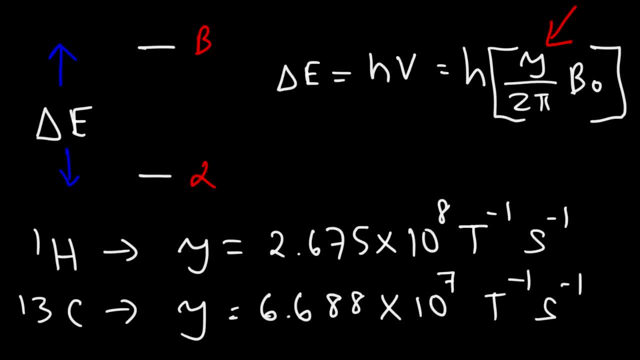 So that's the formula you could use if you wish to calculate the energy difference between the alpha and the beta spin states. Now, sometimes you may need to calculate just the frequency that's needed Given the strength of the applied magnetic field, And it's going to be the gyro magnetic ratio divided by two pi times the applied magnetic. 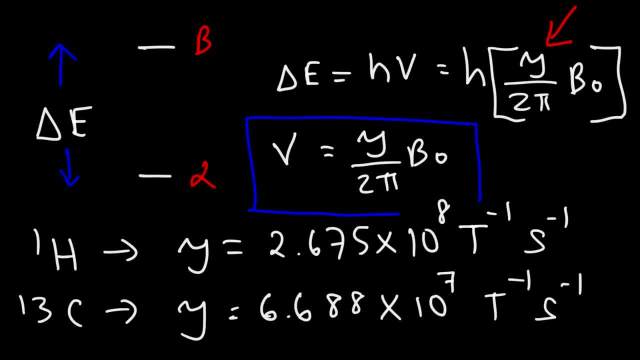 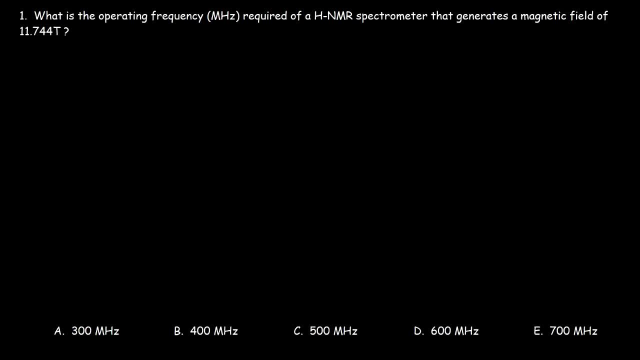 field. So you can also use this formula if needed. Now let's work on this problem. What is the operating frequency required of an H NMR spectrometer that generates a magnetic field of eleven point seven four four Tesla? Okay, So to calculate the operating frequency we need to use this formula.